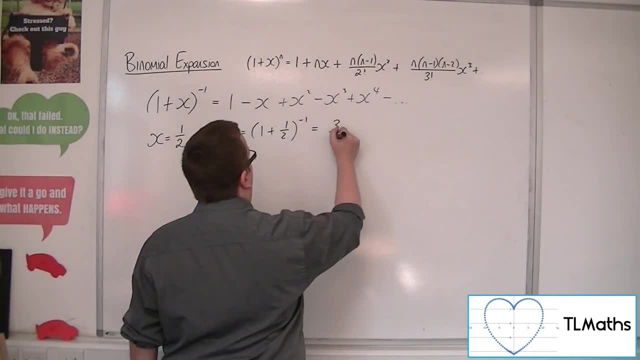 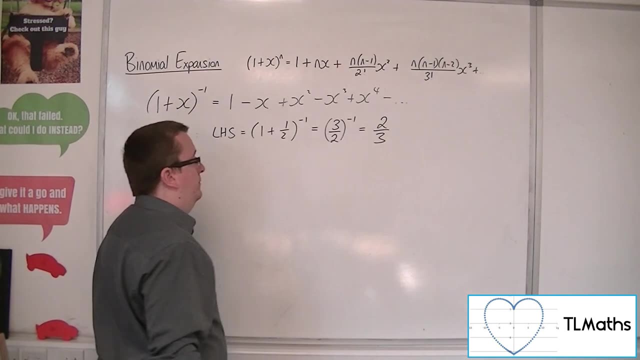 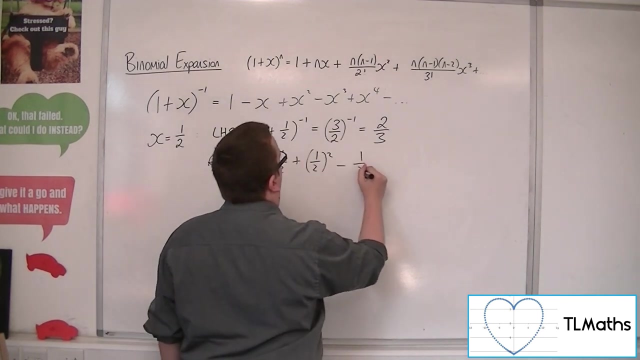 Now, 1 plus a half is 3 halves, And so 3 halves to the minus 1 is 2 thirds. Okay, so that's the left-hand side. Now the right-hand side would be 1.. 1, take away a half plus a half squared. take away a half cubed plus 1 half to the 4, take away a half to the 5, etc. 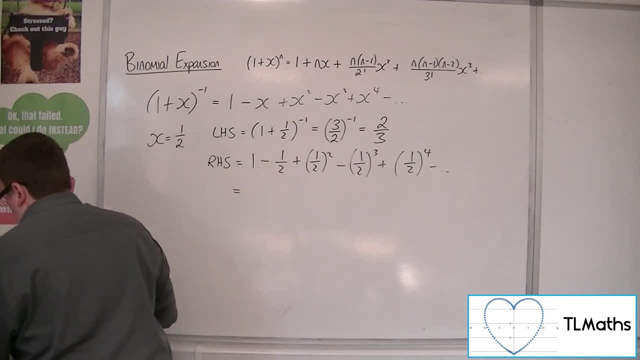 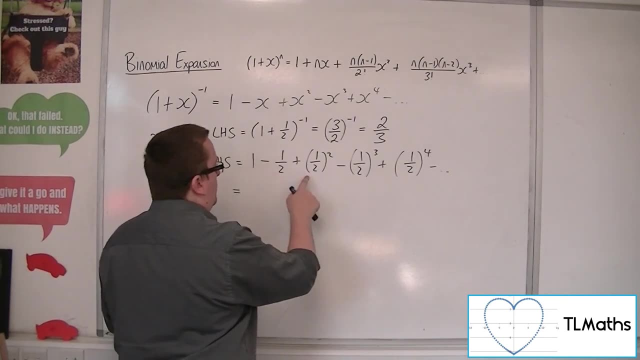 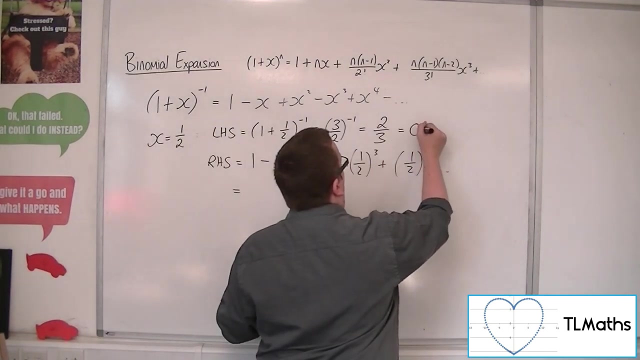 Okay. So if we just do 1, then take away a half, we get 1 half, Okay. Plus a quarter gets us 3 quarters, Okay. So, thinking about this as 0.6 recurring, okay, with those first three terms, we now have 0.75.. 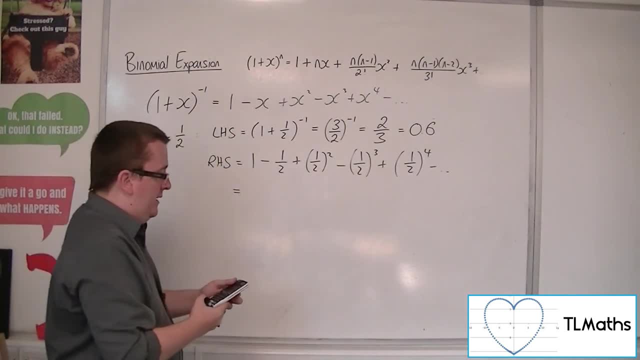 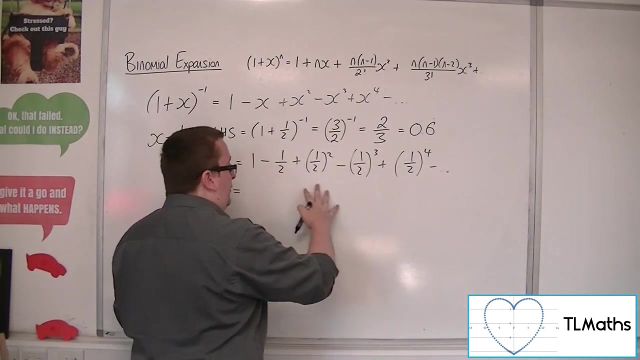 Okay, Take away: an eighth gets us to 0.625.. Then we add on 1 sixteenth, which gets us to 11 sixteenths, which is 0.6875.. So, using those four terms we currently have: 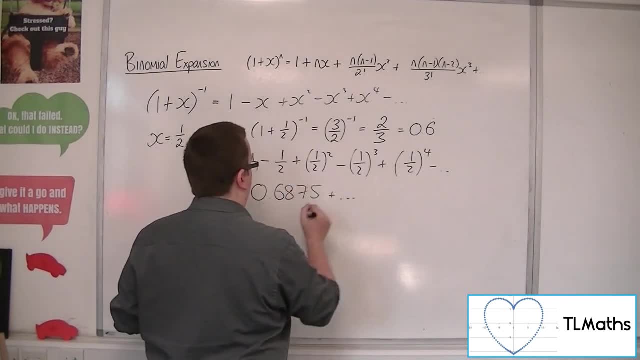 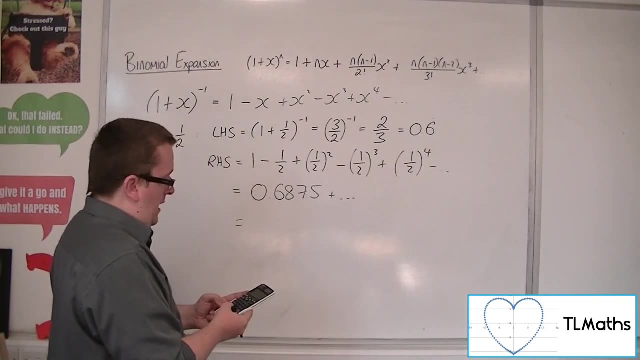 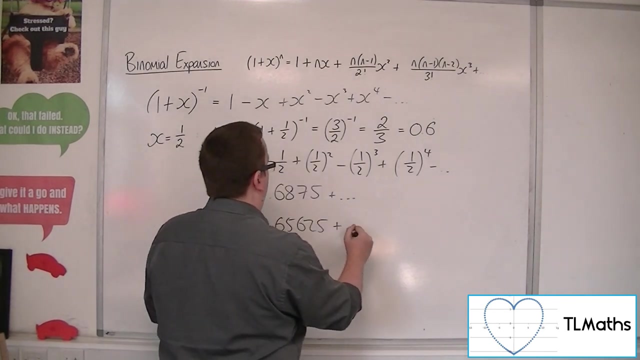 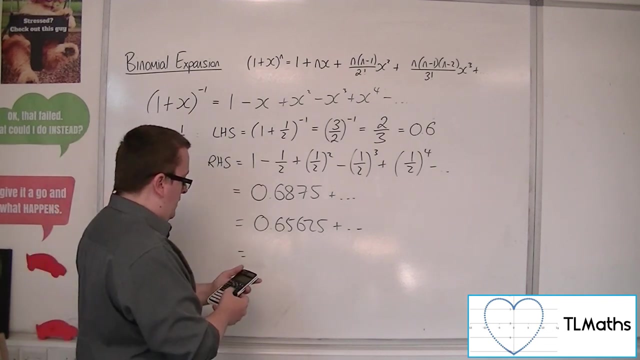 0.6875.. Okay, What if we added on another term? Okay, so we need to subtract 1 over 32 now And we get 0.65625.. Okay, a little bit less. Then I'd have to add on a 64th, which gets us to 0.671875. 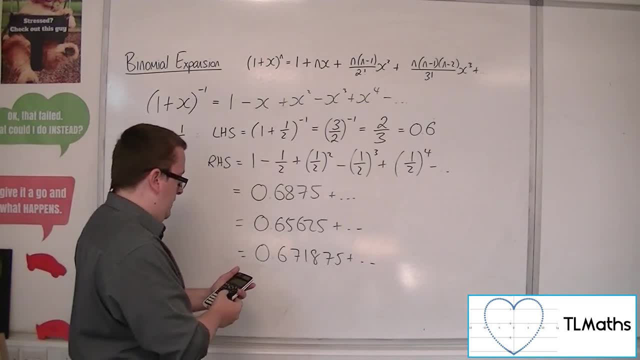 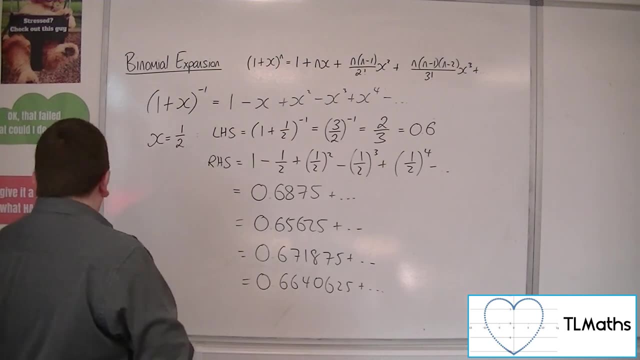 Then I'd have to take away 1 over 128, which is 0.6640625.. So what you can see is that the gaps between these terms are getting smaller, right, And we are homing in on what appears to be 0.6 recurring. 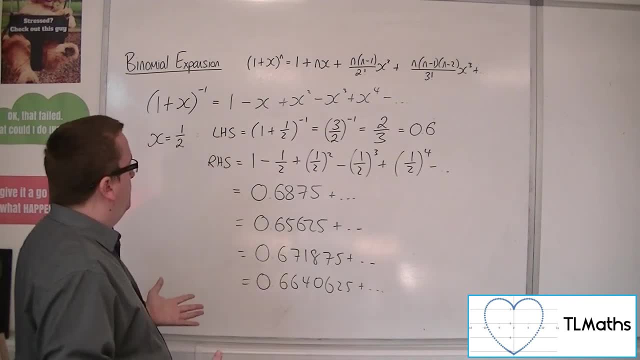 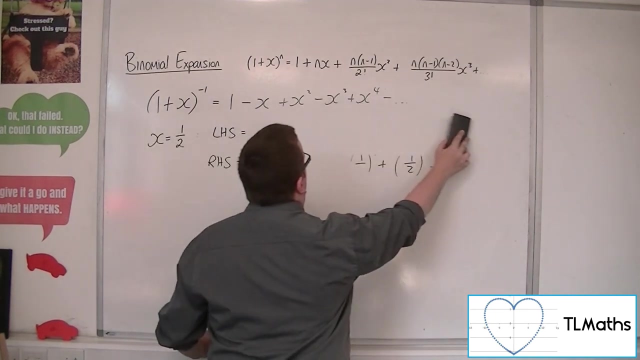 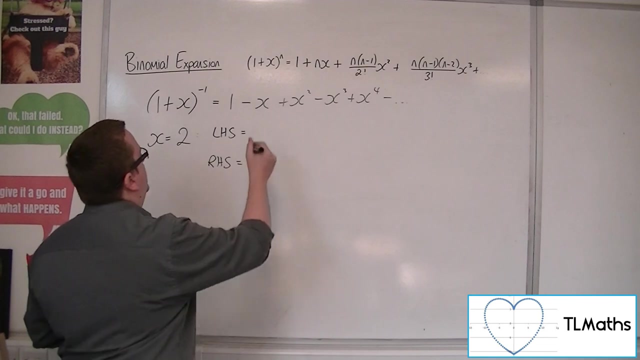 So, just from a little bit of trying it out, x equals a half. seems to work perfectly fine, So what's the worry? So let's try instead. x is 2.. Okay, So the left-hand side would be 1 plus 2 to the minus 1.. 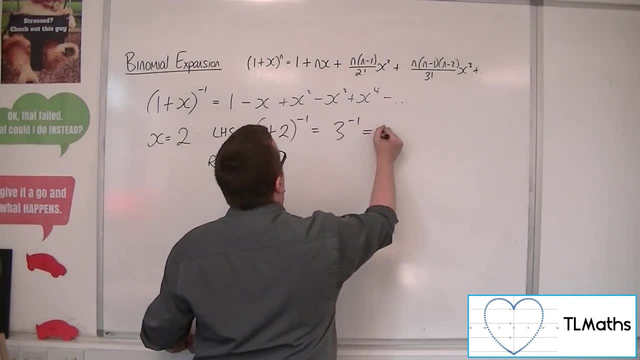 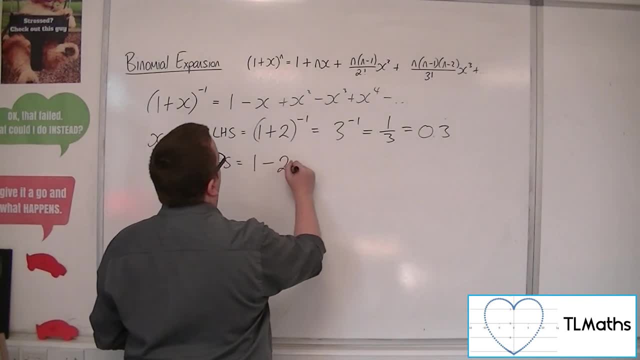 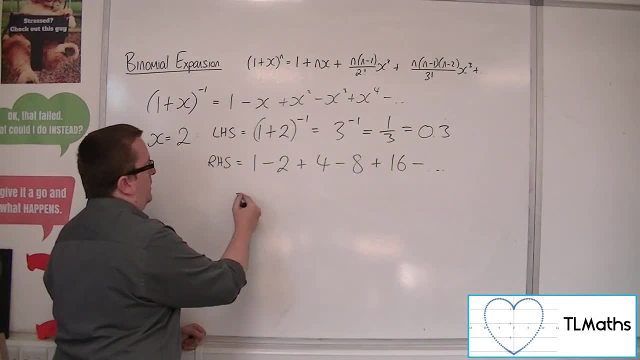 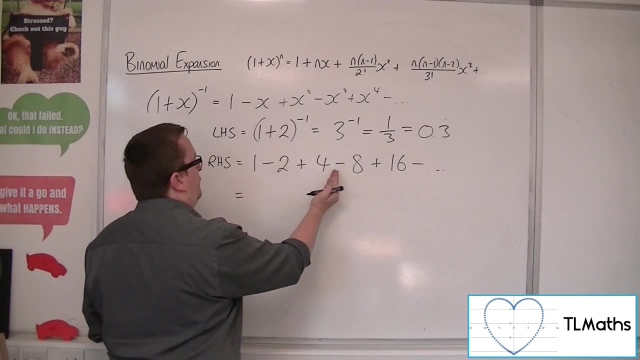 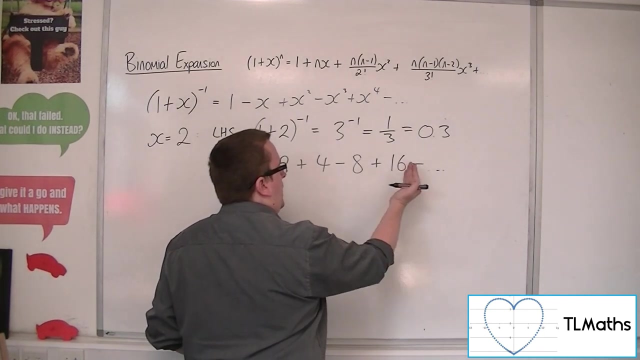 4, take away, etc. Okay, So 1 take away 2 is minus 1.. Add 4, gets you to 3.. Take away 8 is minus 5.. Add on 16, you get to 11.. 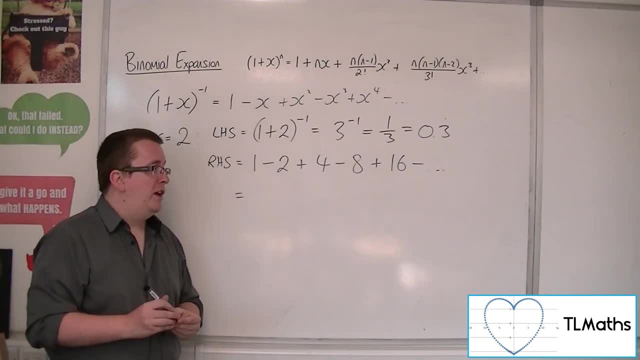 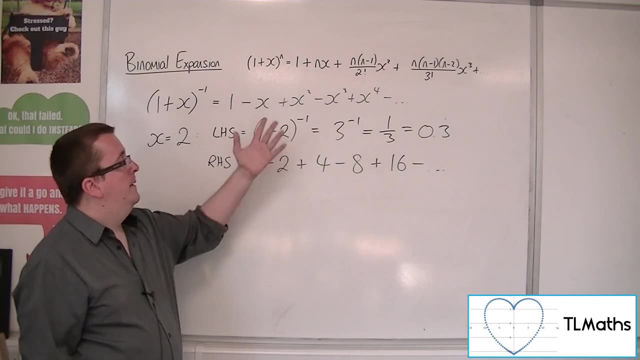 So the more terms we have, the more we lose terms. I'm adding on as I go down this list. I'm actually getting further and further and further away from the 0.3. we're going from the 1 third, and so it's. 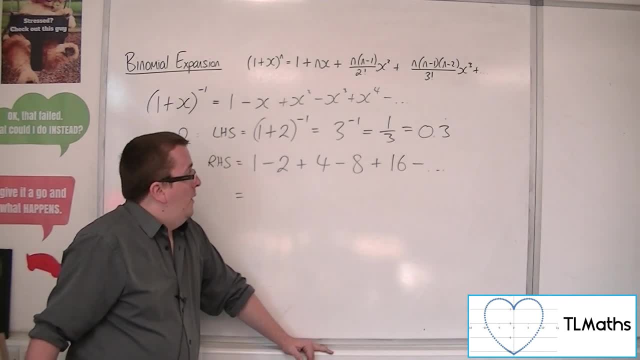 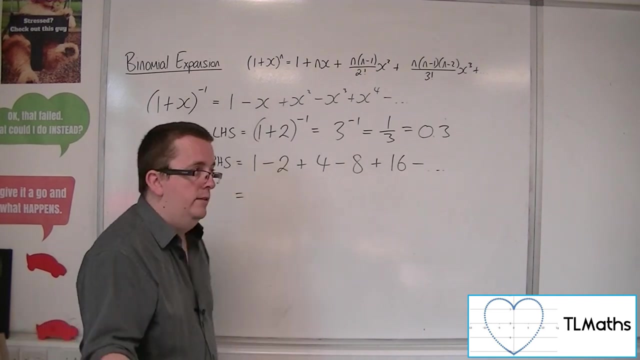 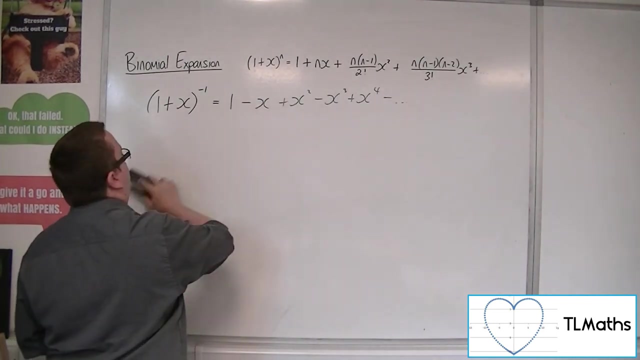 diverging away. so in actual fact it worked for a half, but it didn't work for two. so there appears to be certain values that will work and some that won't, and we refer to this as the range of validity. so what values of X it works? 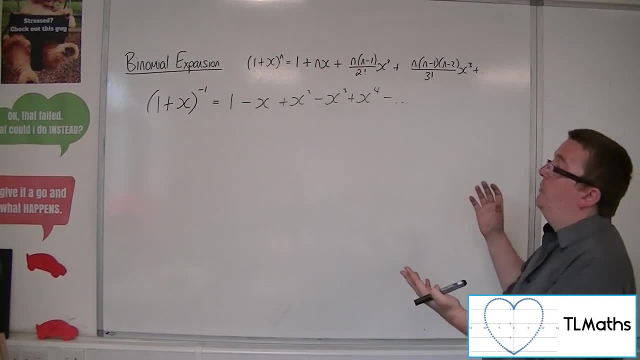 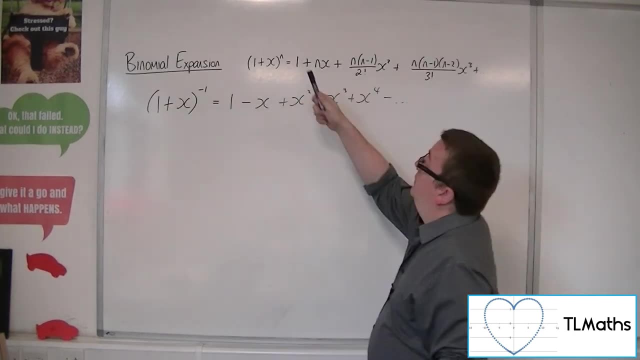 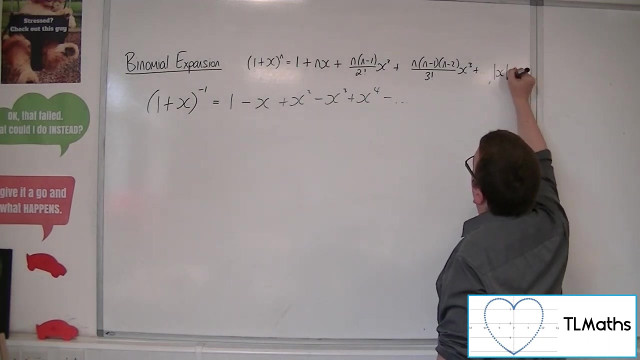 for of it's valid for what values of X can I substitute into the left hand side the right side? I get the same thing. so for this and and for this, this 1 plus X to the n, we must say that the modulus of X must be less. 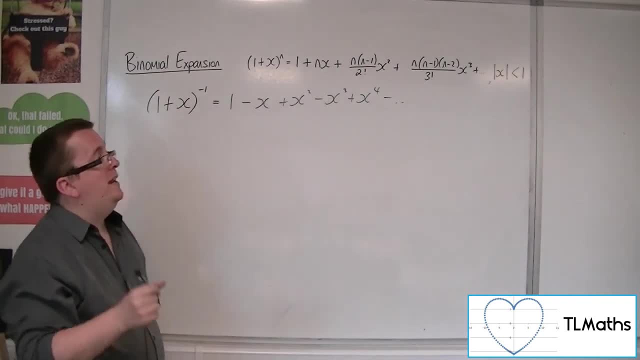 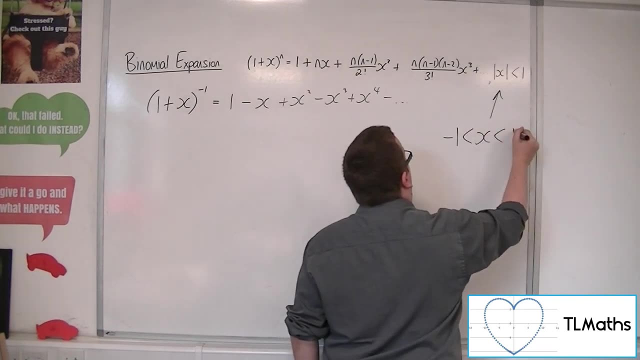 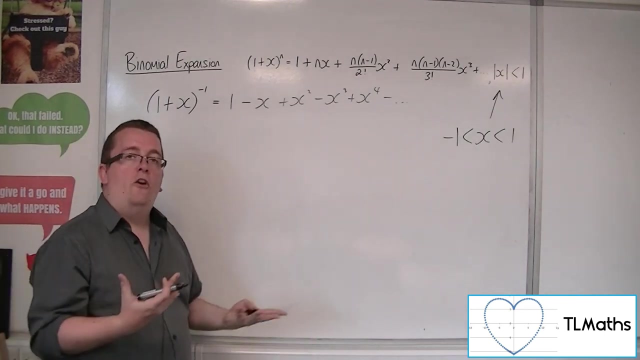 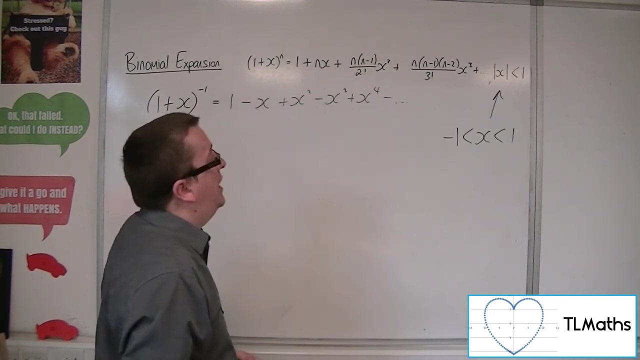 than 1. okay, it only works when X is between, because this is synonymous with saying the X is between minus 1 and 1. if it goes outside of that, then it doesn't work anymore. it's not valid for that, okay. so it requires this concept of the range of validity and we must be able to.